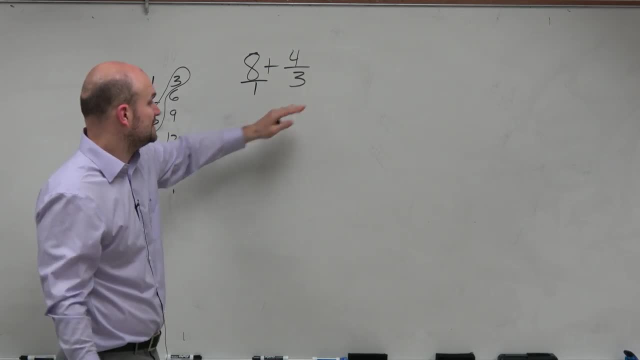 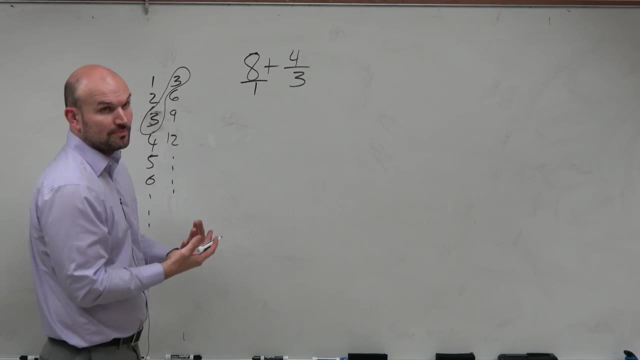 denominators are 3.. Now this denominator is already 3.. So there's nothing we need to do there, But here we need to get this to be 3.. So there's really two ways we can look at this. We could add 2 to it, or we could multiply by 3.. 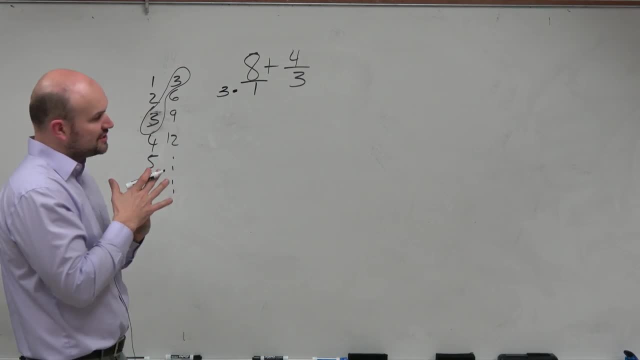 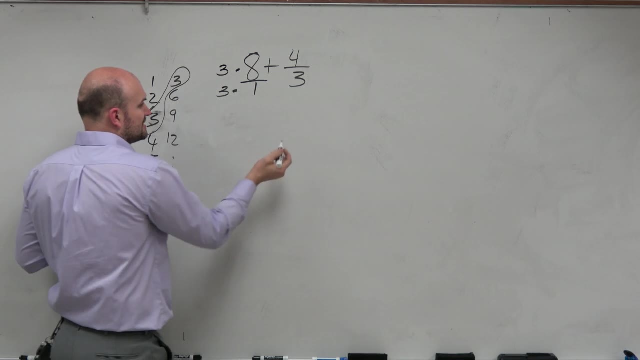 Well, the correct operation is going to be multiplication, Because what that's going to do is that's going to produce an equivalent fraction only if we also multiply by 3 up top, Because, again, just real quick, I'll show you when we multiply. 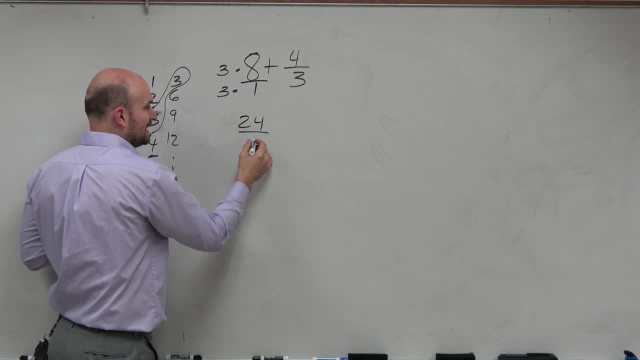 now 3 times 8.. That's 24 over 3 times 1 is going to be 3.. 24 over 3, or 24 divided by 3, is the same thing as 8, right 3 goes into 24, 8 times. 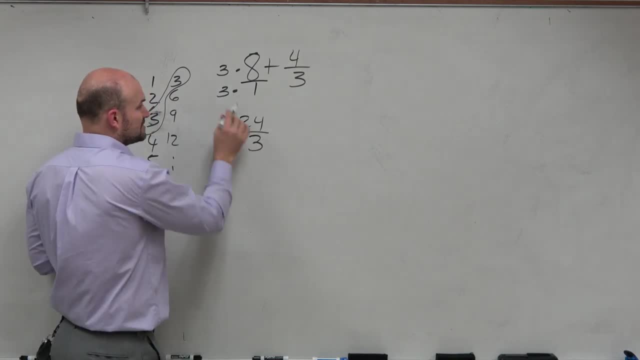 Now let's just pretend that we added 2 instead. So therefore let's say we added 2 in the top and the bottom, So therefore we'd have 10 thirds. 10 thirds is not equivalent to 24 thirds, right? 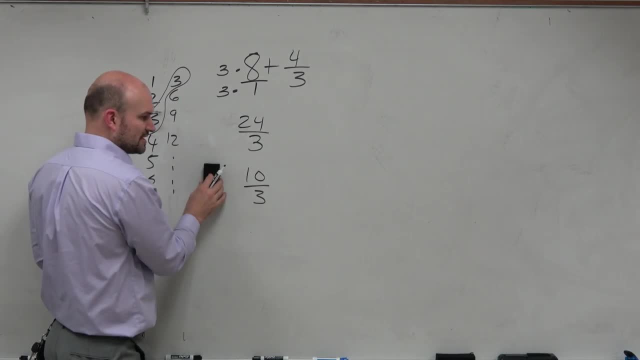 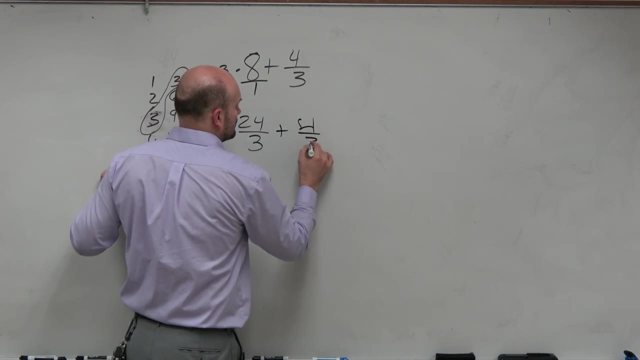 Those are not the same fractions. So that's why adding is not going to work. It's not going to produce an equivalent fraction. So we're going to multiply by 3 over 3.. And now we don't need to do anything to that fraction. 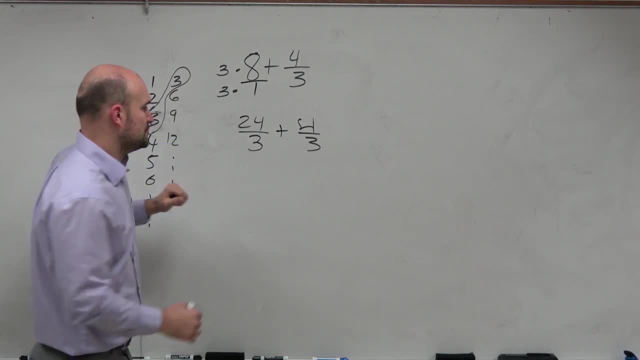 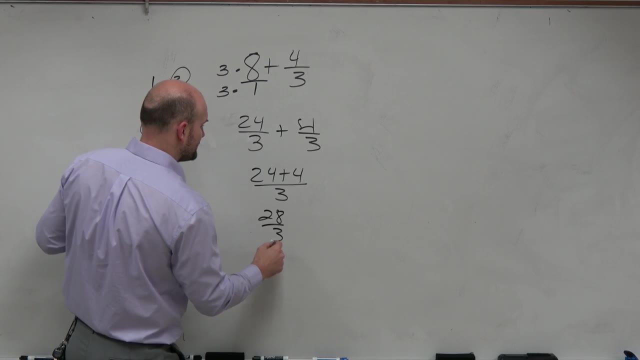 Now we have the common denominators And now we can just apply our operation to our numerator. So basically we're just going to add 24 plus 4 over 3.. 24 plus 4 is 28 over 3.. 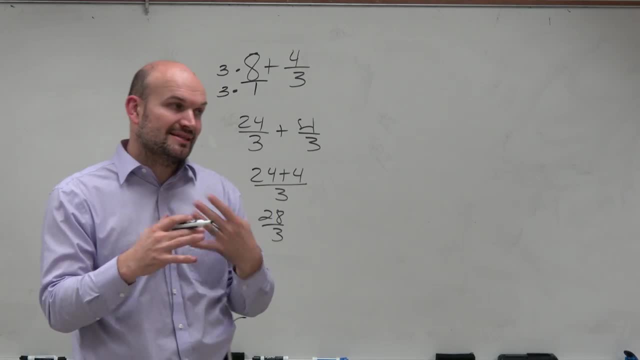 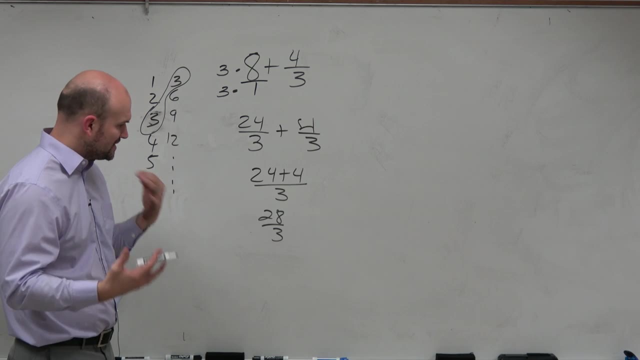 Now the next thing we'd want to do is go ahead and see if we need to rewrite this as a mixed number. I prefer to leave it as an improper fraction, However, for some classes or teachers or tests and quizzes. 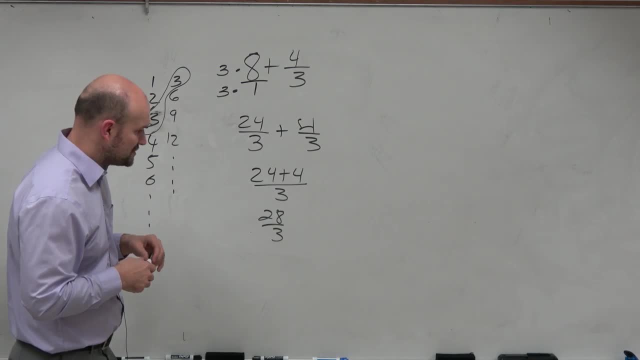 or whatever might need to go ahead and rewrite this as an improper fraction. So to do that, You're going to say: how many times does 3 evenly divide into 28?? Well, 3 times 9 is 27.. And 28 minus 27 is 1.. 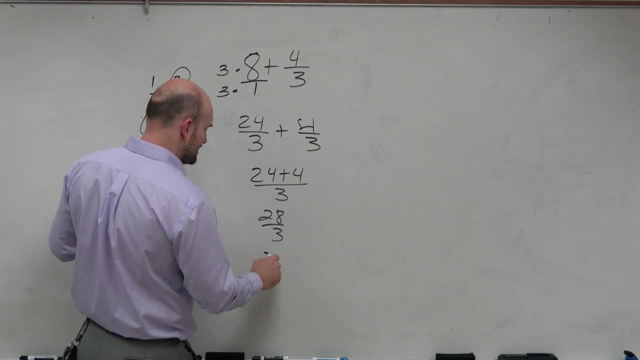 So that means as a fraction. we could write this as it goes in there 7 whole times. right, 3 goes into 7, not 7 whole times. It definitely goes in there 7., But you say it goes in there 9 times. 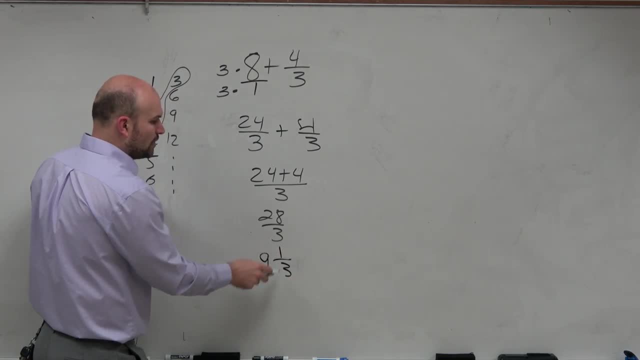 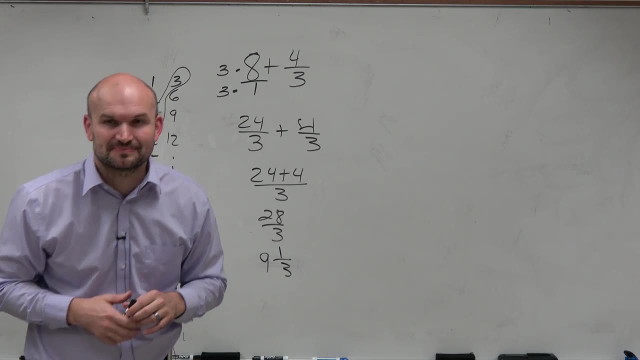 and with the remainder of 1.. So, really, 9 and 1 thirds is equivalent to 28 thirds. So there you go, ladies and gentlemen. That is how you add a whole number to a fraction. Cheers.